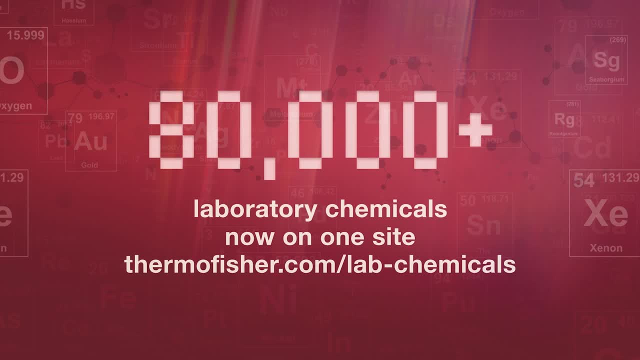 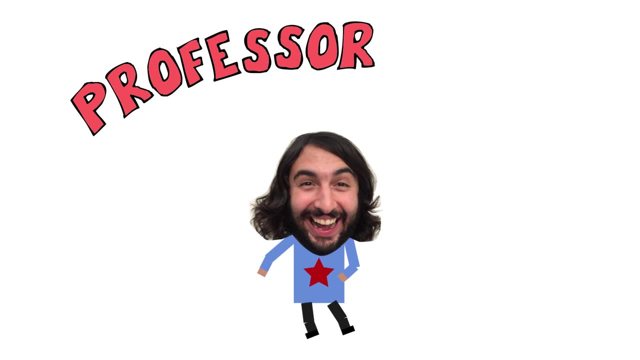 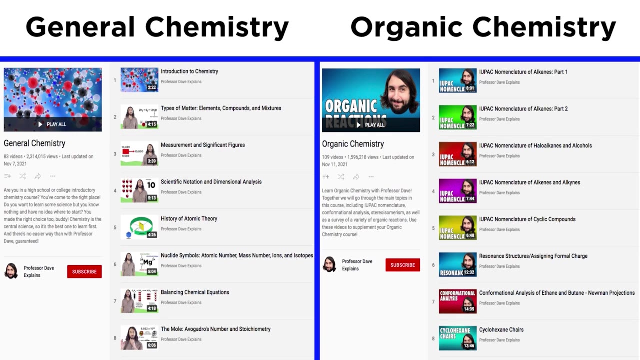 site. Thermo Fisher delivers choice, quality and supply assurance for all your chemical needs. Visit the link below for more information. We have learned a lot together on this channel regarding general chemistry and organic chemistry, but we have focused predominantly on concept-based learning rather than practical knowledge, While 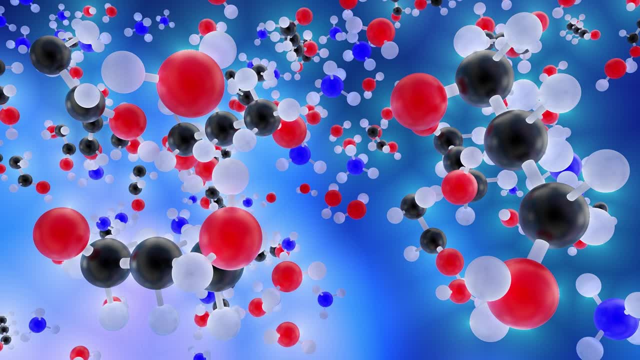 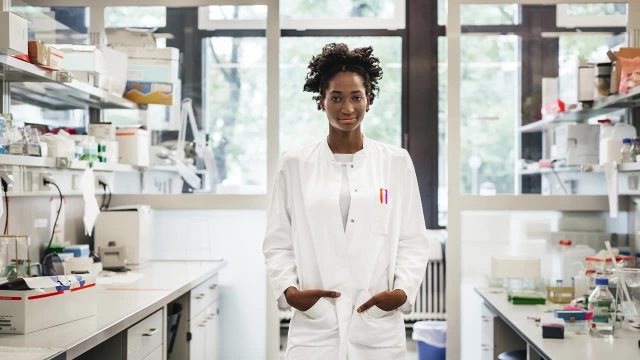 it is certainly extremely important to understand what molecules are and how they behave on a conceptual level. one can never have a true understanding of chemistry until they get into the laboratory and learn about it. If you're interested in learning more about chemical chemistry, please subscribe to our channel, and don't forget to hit the bell icon so you don't. 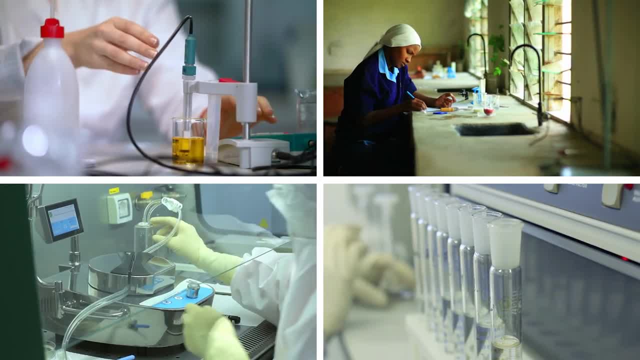 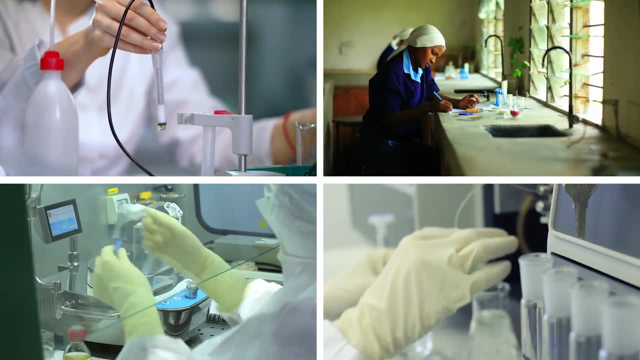 miss out on any of our future videos In this series. we will take the chemistry we have learned together and see exactly how it can be applied in order to do empirical science. We will learn how to perform chemical reactions, as well as a variety of analytical techniques. We will 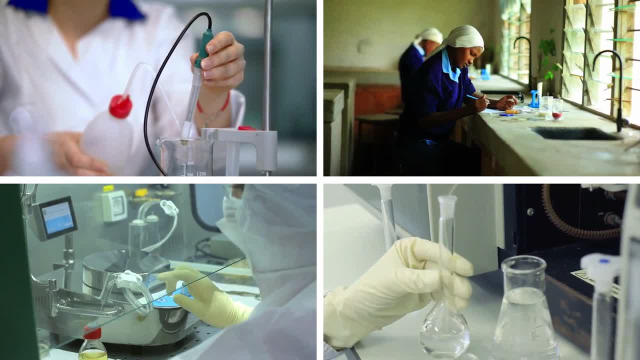 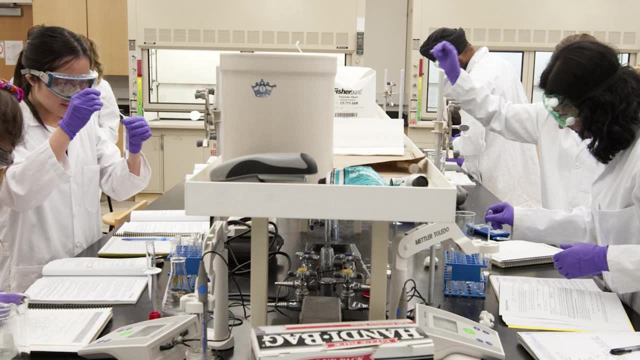 learn how to interpret data and solve problems. Since doing chemistry requires a wide variety of specialized instrumentation, this series will be most useful for undergraduate students and advanced high school students who are taking chemistry courses with laboratory components for the first time. Together, we will discuss the most commonly performed techniques in such courses. 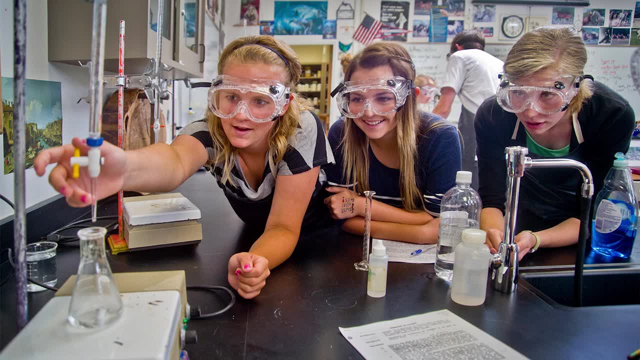 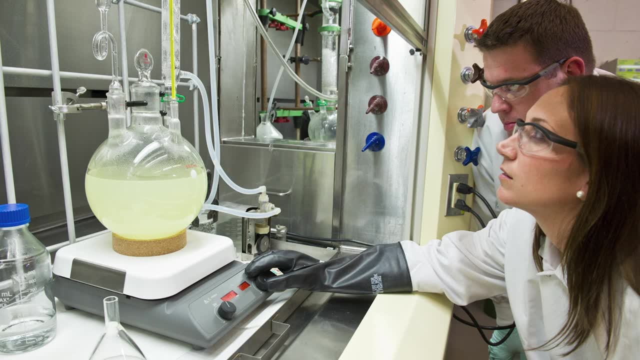 so that you can approach your assignments with clarity and confidence. But even those who are not formally studying chemistry may find this series worth watching, as it is fascinating to learn about the precise methods we use to discern knowledge about the molecular world. How can we? 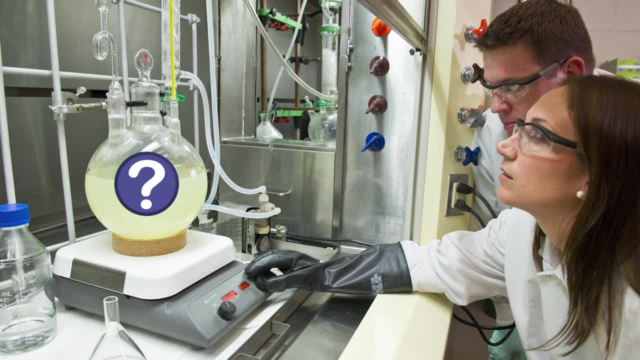 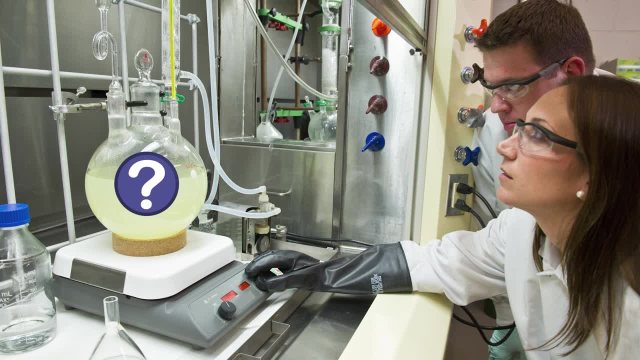 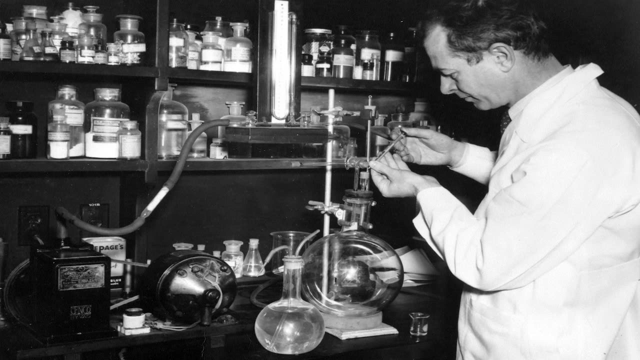 finished. How do we perform chemistry that is air-sensitive? Once a competency in the laboratory is gained, a grander context for chemical knowledge opens up like an oyster, and an appreciation for the astounding contributions of the chemists who came before you becomes apparent. Whatever your 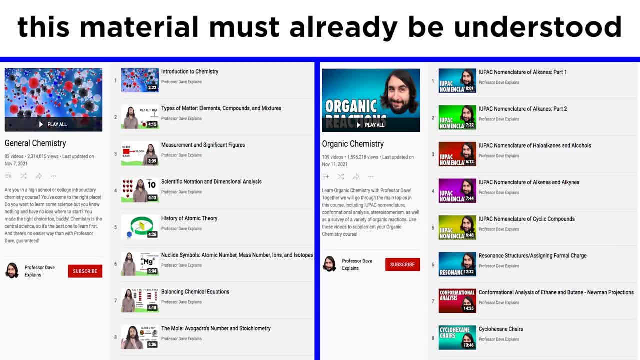